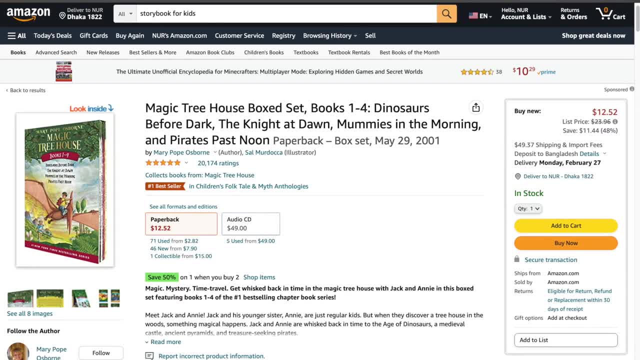 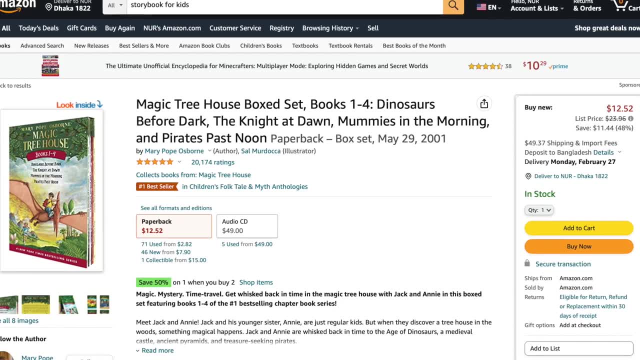 ideas for my business. Then I found this product, which is a storybook for kids. You might say, okay, what's interesting about it? After doing my research, I was shocked by the number these sellers make by simple storybooks like this. As you can see, this book got 20,174 ratings and 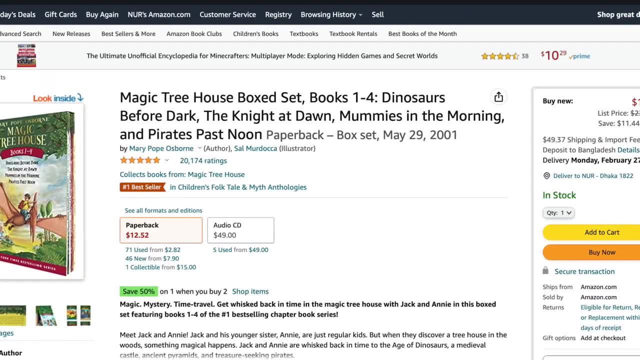 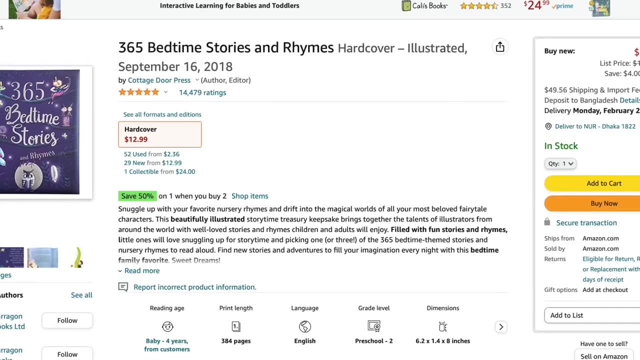 if we multiply that by 12.52, which is the product price, you'll find out that the seller has made over $252,000 from this book. So if you are interested in making passive income, keep watching alone. Let's see another one. This book got over 14,479 ratings. multiplied by 12.99, that will be: 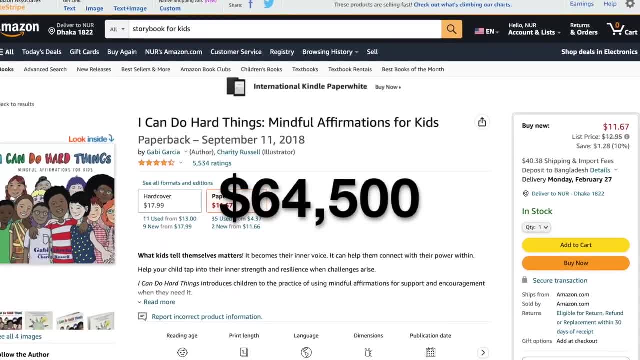 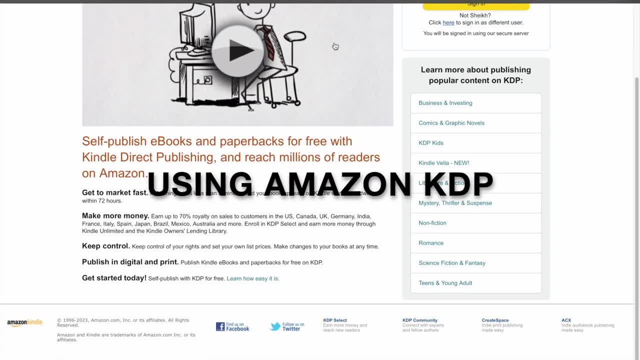 over $188,000 and this one has made over $64,500.. The craziest is that you can publish these books 100% free using Amazon KDP. Then I said: okay, why not create a similar book using chat PT? 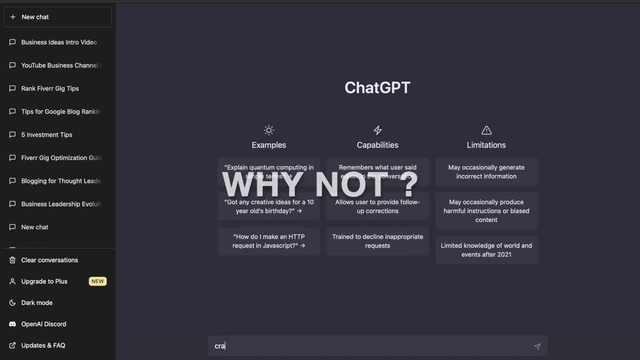 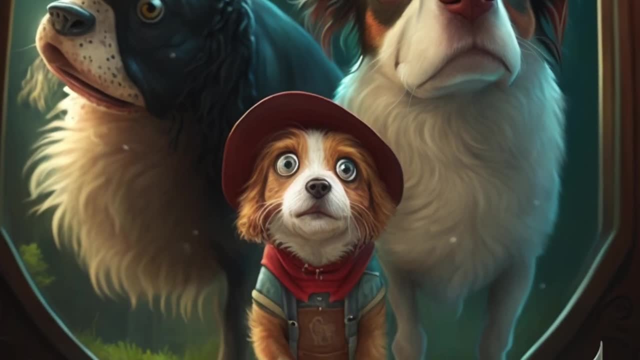 publish it on Amazon and generate a passive income that makes money while sleeping. So I decided to make this video to help as many people as possible. As you know, to create a good storybook, you first need to come up with a good story idea. 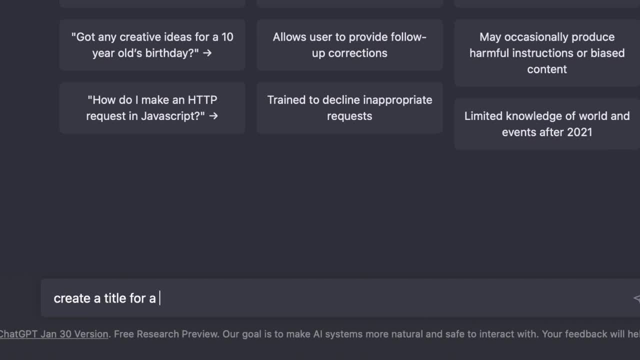 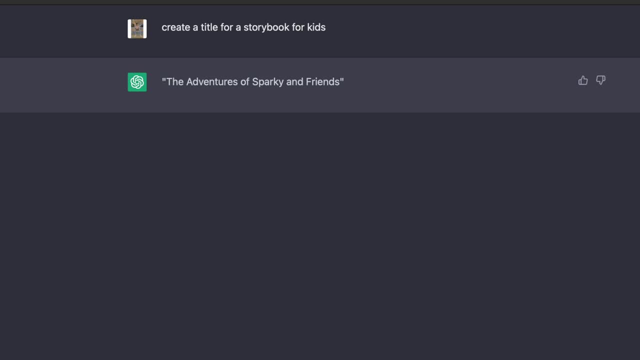 So I asked the chatbot to generate a title for a storybook related to kids And the answer was The Adventure of Sparky and Friends. Okay, that sounds like a very exiting story we can work with. Then I asked the chatbot to give me more details about the story, and it came out that the book is 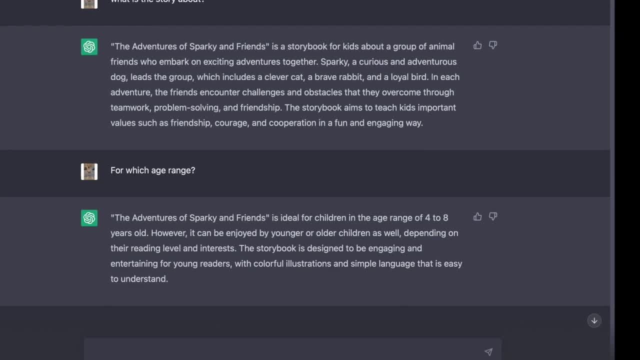 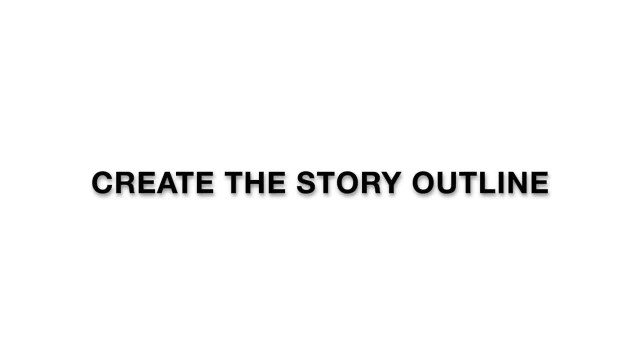 for kids between 4 to 8 years old, and it is about Sparky and his friends, who embark on exiting adventures together. I really liked the idea, so I decided to move on with this one. The next step was to create the story outline. As you can see, the chatbot has generated the chapters and each. 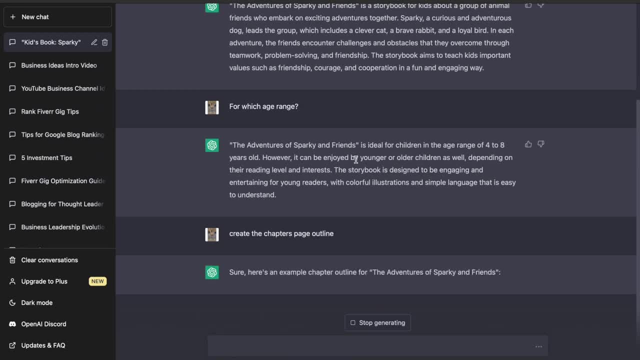 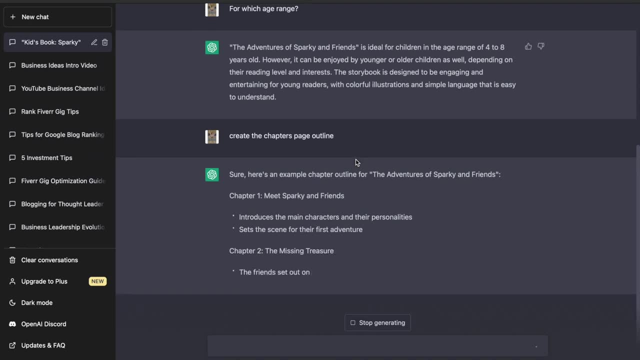 chapters include the scenes in detail: Chapter 1, Meet Sparky with his friends, Chapter 2, The Missing Treasure, And we got 8 chapters in total. Now that we've generated the story outline, now we can start creating the actual story content based on the chapters. All you need to do is copy. 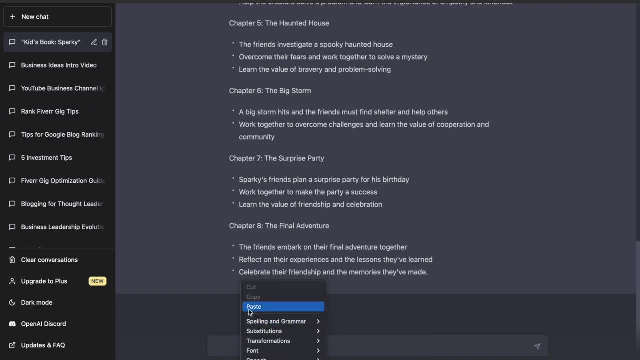 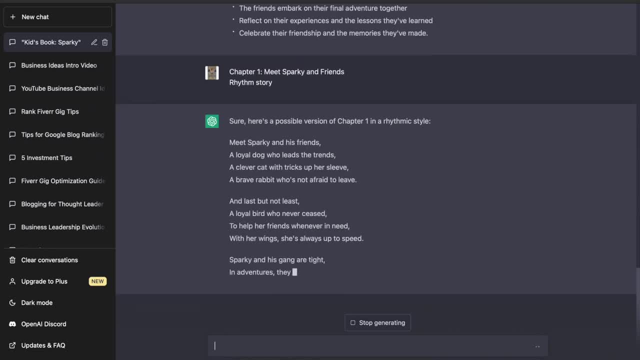 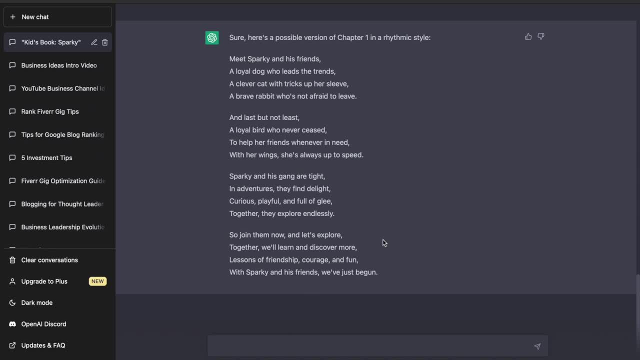 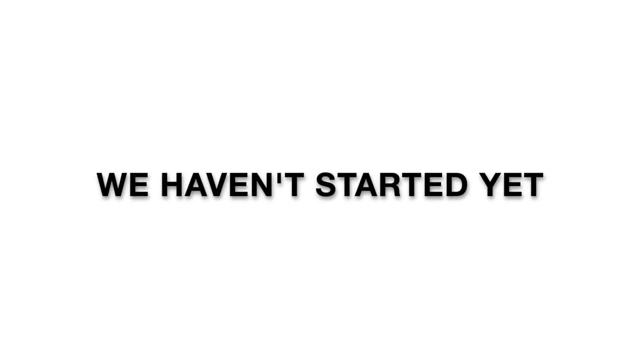 passive income without needing to write anything myself. If you think about it, it's actually crazy how fast we came up with the story idea and chapters, along with the story content. But trust me, we haven't started yet, Because what comes next is mind blowing. So if you enjoyed the video, so 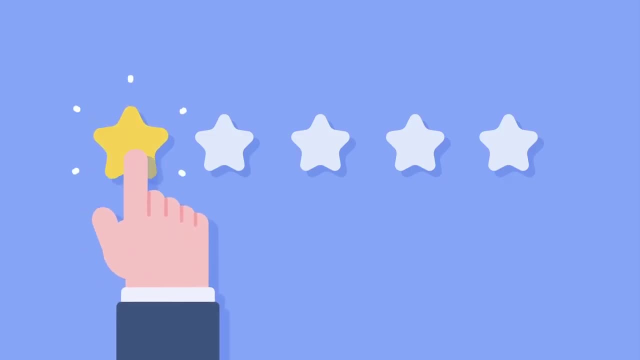 far, hit the like button. We all know that even if you have the best story idea, it won't be good enough for you. So if you enjoyed the video so far, hit the like button. And if you want to see, 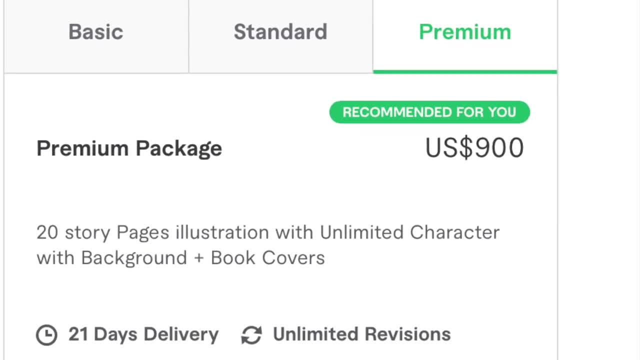 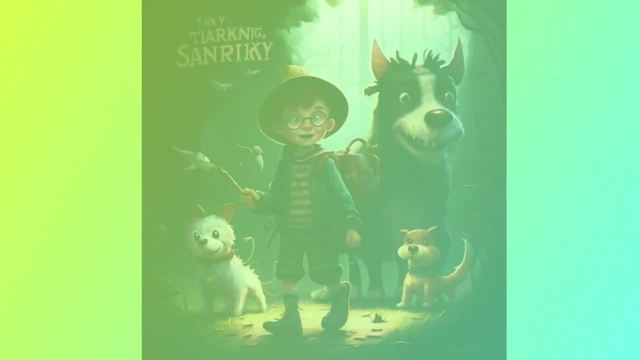 it again. hit the subscribe button And here you could easily pay thousands of dollars for artists to finish these illustrations. But what if I told you that all images you see on the screen were generated using an AI art generator for 100% free? Would anyone believe that? You surely heard. 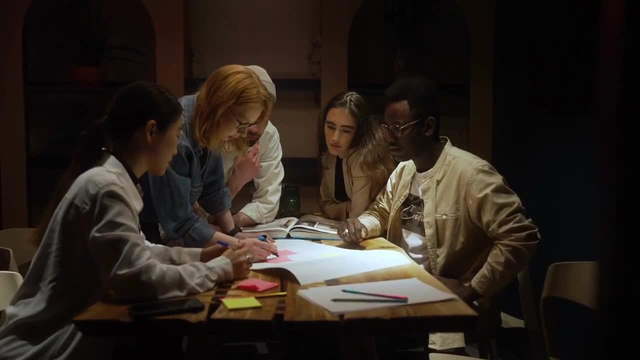 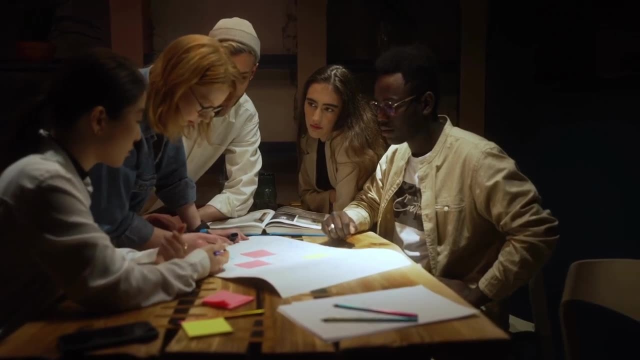 of AI art and how you can generate original images by typing some words, And this is what I did to finish my first chapter of the story. Let me show you how, When it comes to AI art generator, there are many options available. I've tried a lot of them and I found that Midjourney provides the best. 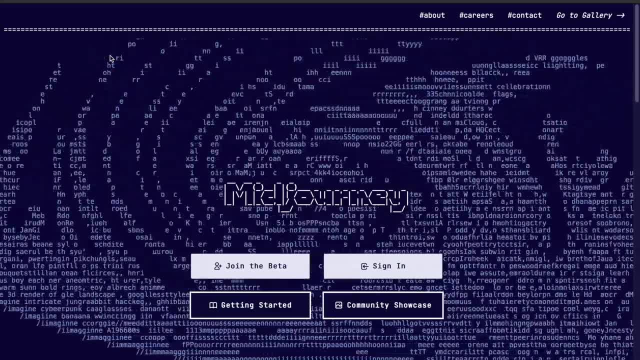 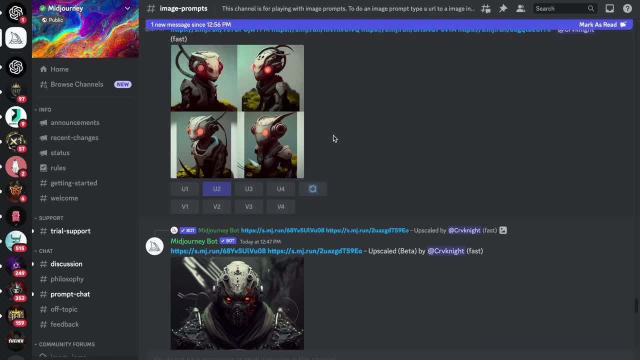 experience and the best experience. So if you want to learn more about how to create an AI art, in my opinion you can try it for free using the link below this video. Once you've joined their Discord server, you can see all recently generated images. There are millions of users, So you will. 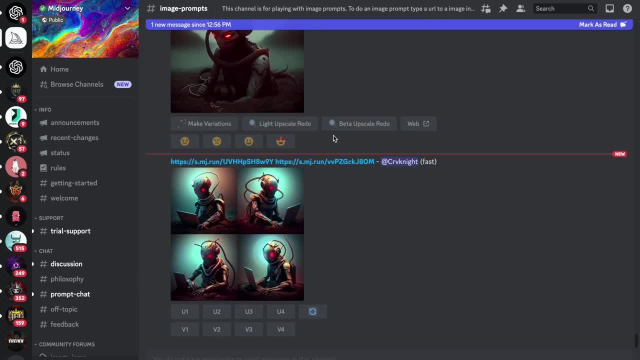 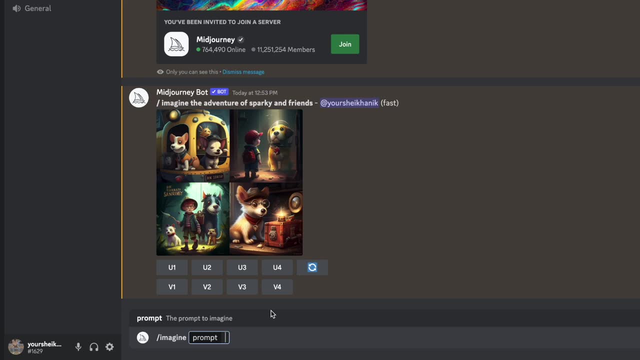 notice that new images are generated every second. To generate your image you need to start a prompt. First type forward slash and then imagine. Once you do that, you can start explaining the image you want to generate. Go back to the story chapters you've generated before and copy the 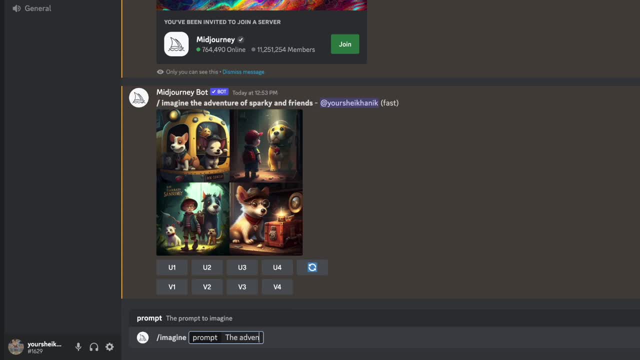 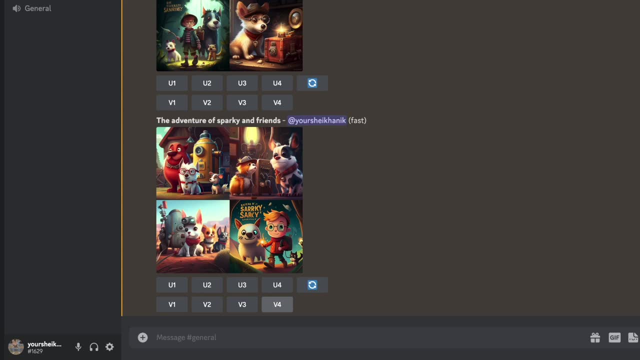 first one, In my case it was meet Sparky with his friends. So now we the image we want to create. So again, we type forward, slash, then imagine and then your chapter topic. After the image has finished generating, two rows of buttons will appear, As you can see, in the top row: U1, U2,. 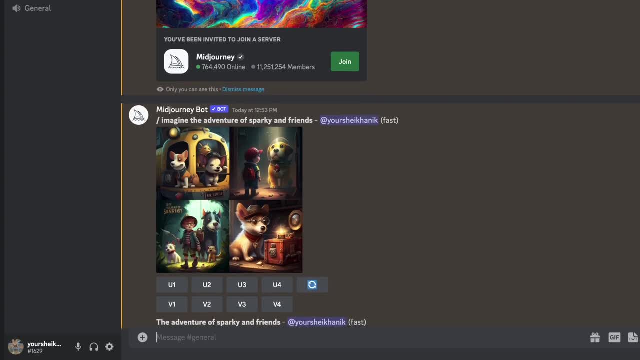 U3, and U4.. These buttons are for upscaling your chosen image, which means generating a larger version of it In the bottom row. V1,, V2,, V3, and V4.. These buttons create four new variations, similar style and composition to your selected image. So to recap, if you click U1, it will. 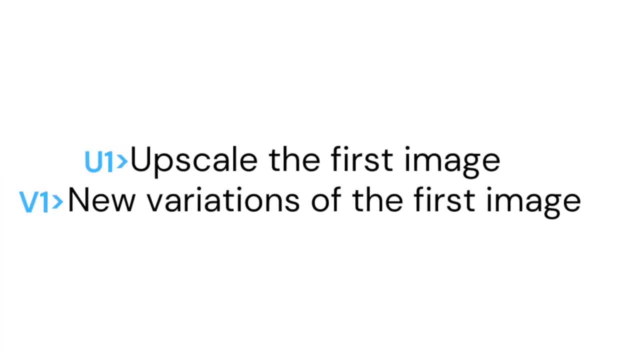 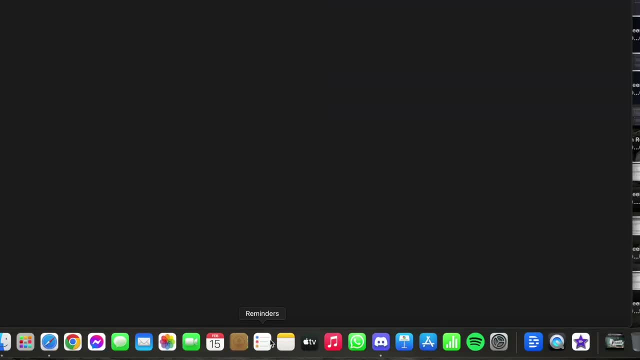 upscale the first image and clicking on V1 will create new variations. So to recap, if you click new variations of the first image, In my case I like the first image, So I clicked on U1 to make it bigger. To save the image, right click and then open link. After that right click again and save. 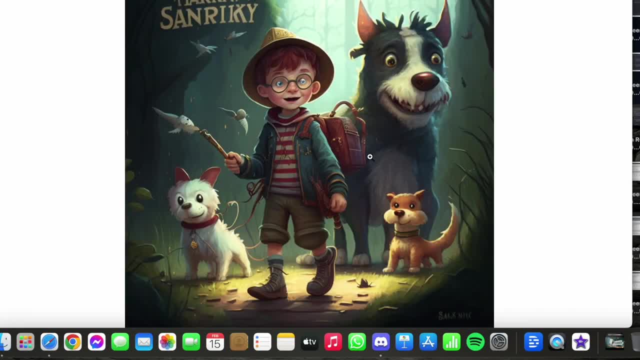 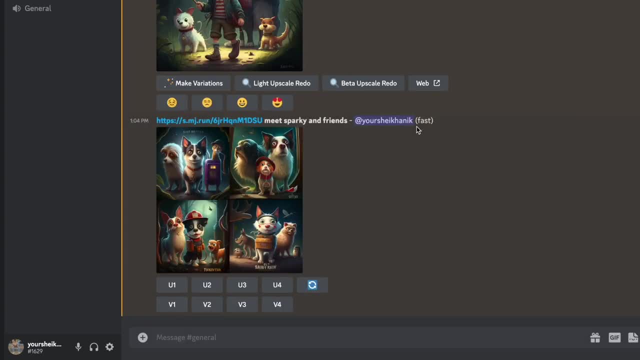 it to your device. Then you will create all the images you need, like this To keep the same style. here is a simple tip: Copy the first image link, start the prompt and paste the link before explaining the new image. That way you can maintain the same style. I like the second. 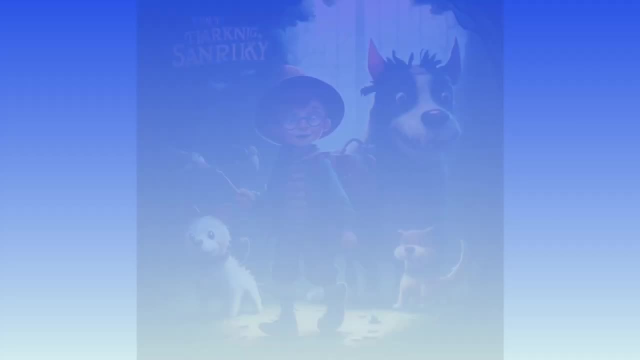 version. So I clicked on U2 to upscale, Then I did the same to all images And in about 30 minutes I had the illustrations ready to use. I won't repeat the process for all the chapters cause the video will be too long, but you got the idea: Start section by section and generate the images. 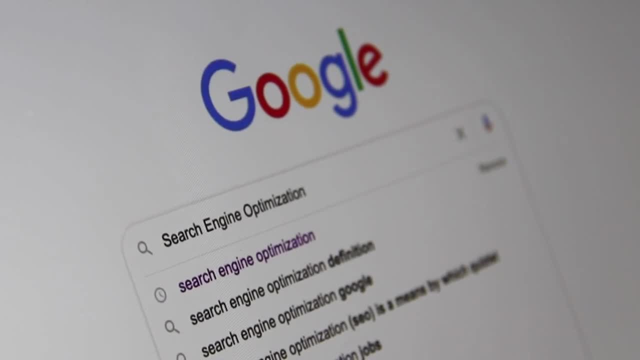 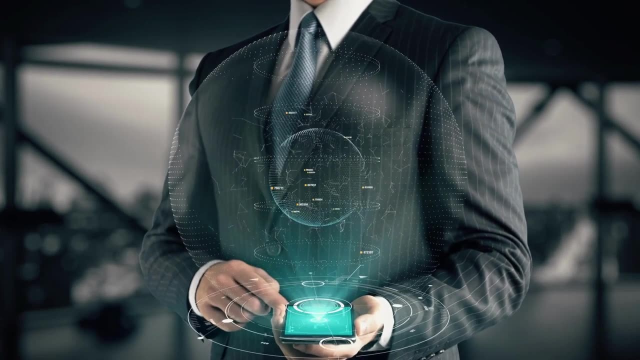 based on your story topic. If you still need more help using Midjourney, I'll leave a detail guide below this video. Now that we've generated the images, let me show you how to combine the text generated using ChatPT with the images generated using Midjourney to create a professional looking. 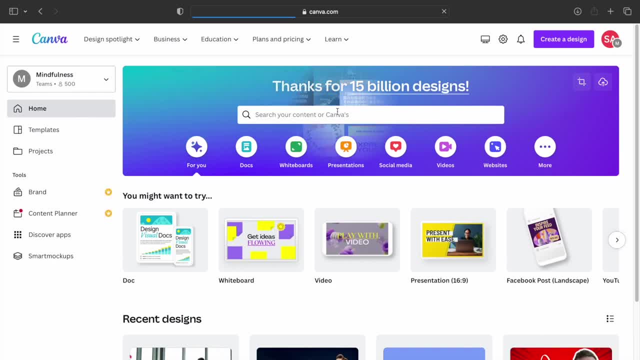 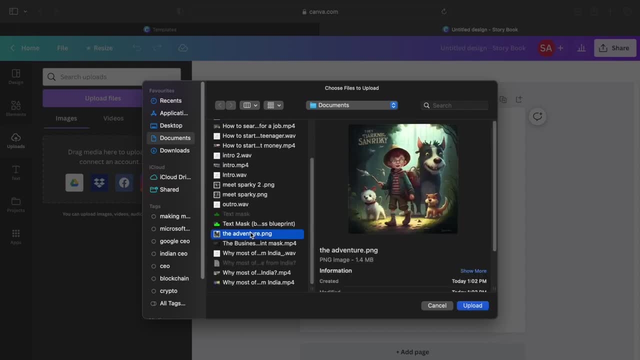 storybook. First hit to canvacom and search for storybook. then click on create a blank storybook. After that, start uploading the AI generated images to Canva. Then you can simply drag and drop the first image into the template. Now go to ChatPT, copy the first part of the story and 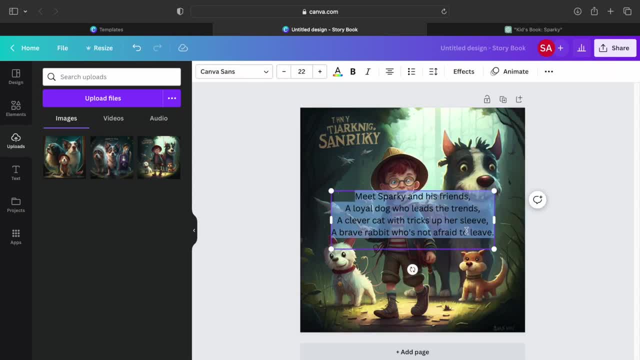 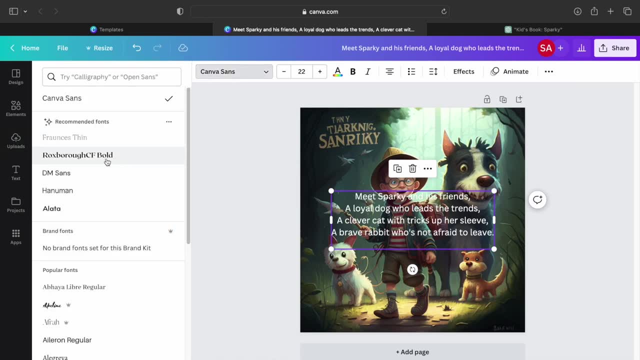 paste it on top of your image. You can now adjust the text as you like. You can change the color, the font style, add shadows. I really like Canva because it's beginner friendly and it doesn't require any design skills and top of that, it's free to use When you're done. click here to 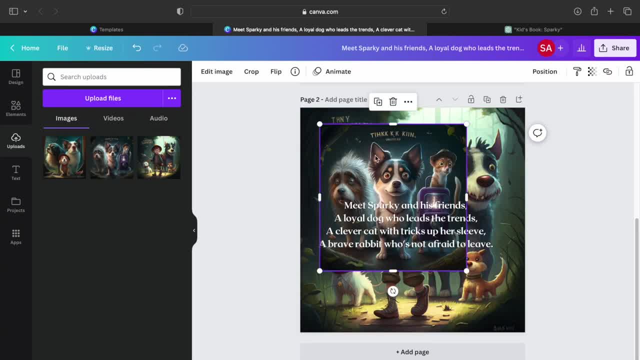 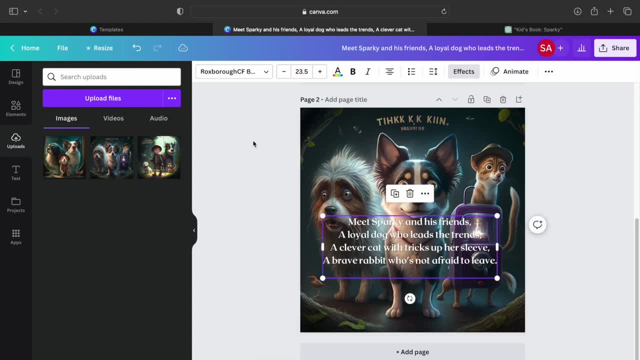 duplicate the template. Doing that will save you a lot of time, Because now you can add the new image, style remains the same. After that, all you need to do is duplicate the same process in all the chapters of your book and, once you've done, save the book as a PDF print. Congratulations, you've. 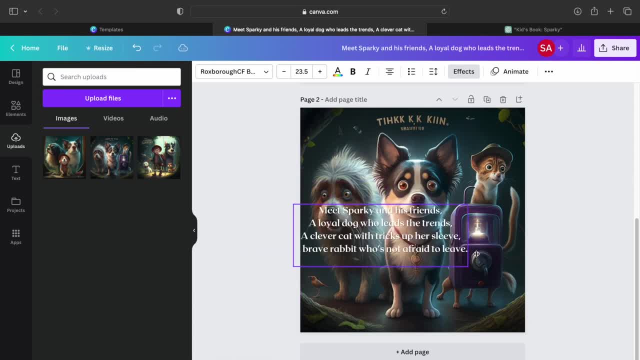 created your very first storybook successfully and there's only one step left to start making passive income, which is publishing your book on Amazon. Unfortunately, I won't be able to explain the entire process because this might take another hour, but instead I have left a step-by-step guide.